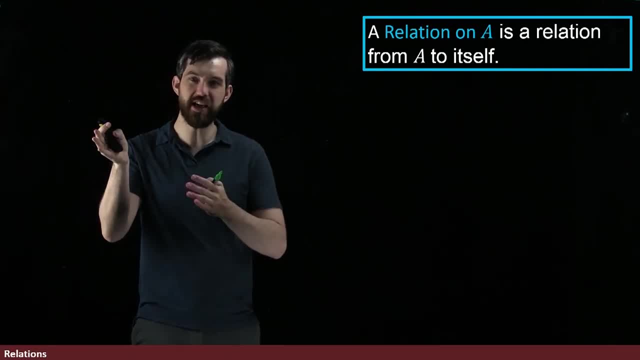 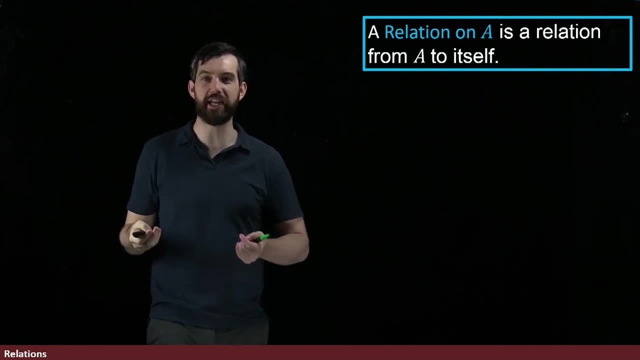 I could also consider relations not from an A to a B, but from A to itself. This is perfectly valid. For example, we see relations or functions from, say, the integers to the integers all the time, So I can refer to a relation on A. But how should I think of this? How should I sketch this? Well, 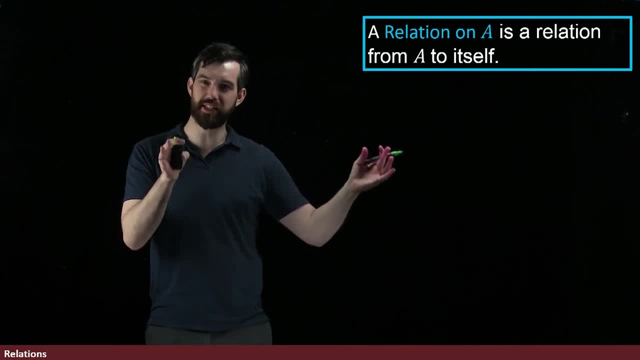 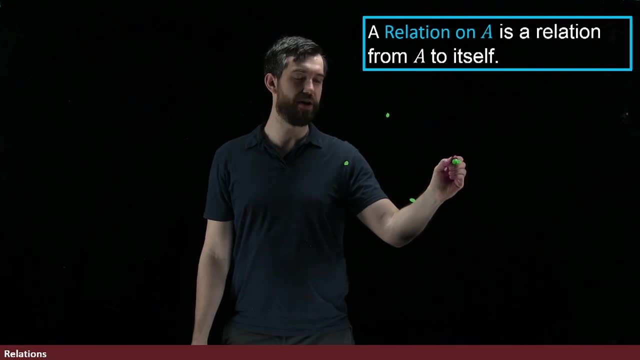 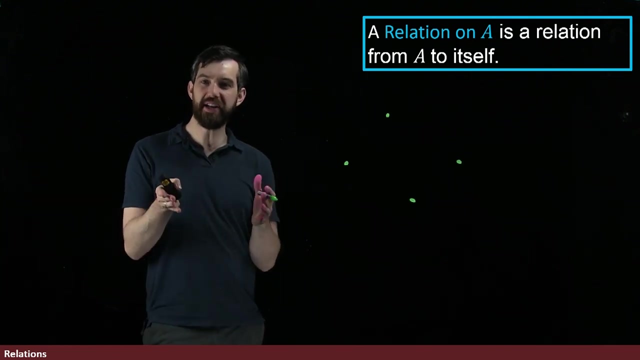 I don't have a domain and a codomain exactly, or at least the domain and the codomain are the same thing, So I'm only going to draw one. So how would I start? by putting a collection of points down. So these are just some points that are going to represent the elements of A And then one way. 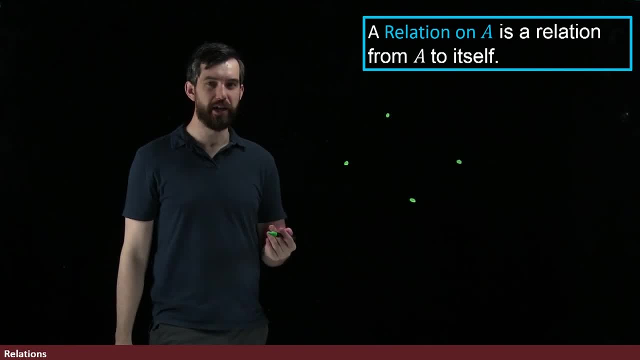 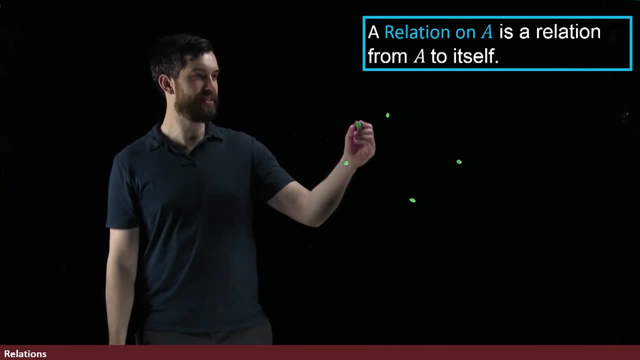 to think about a relation was as an arrow diagram. So you took elements in your domain and spat out elements in your codomain. So what I'm going to do here is I'm going to take an element- how about like this one, and where does it go? And I'm going to draw an arrow to somewhere. And this time 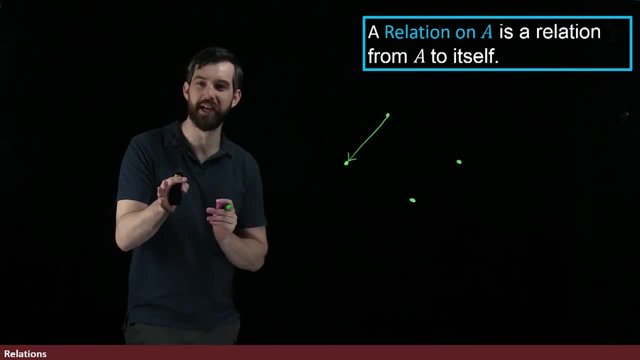 I really do care about putting an arrow in, because we can't use the trick that the domain and the codomain are on the left and the right, So we have to indicate where I'm starting and where I'm finishing. So when I draw an arrow I say I'm starting at this point and I'm finishing over here. 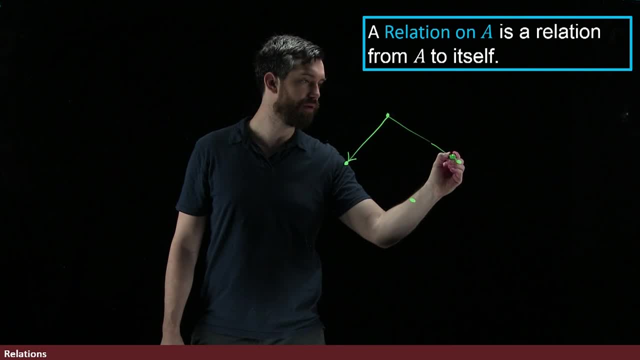 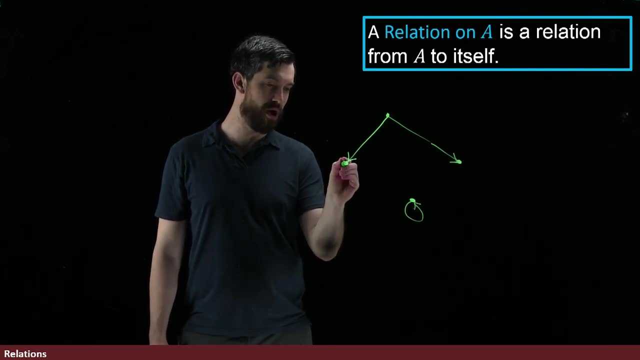 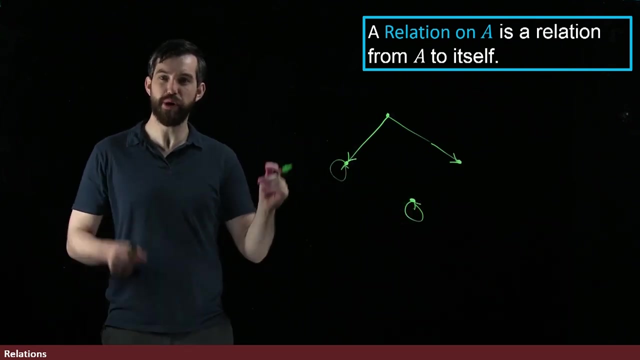 Maybe I start at this point and I finish over here, And maybe I start at this point and then I finish right back at itself, And maybe this one loops around back to itself as well, This kind of construct that I'm drawing, where I put my points and then I draw arrows between those points which 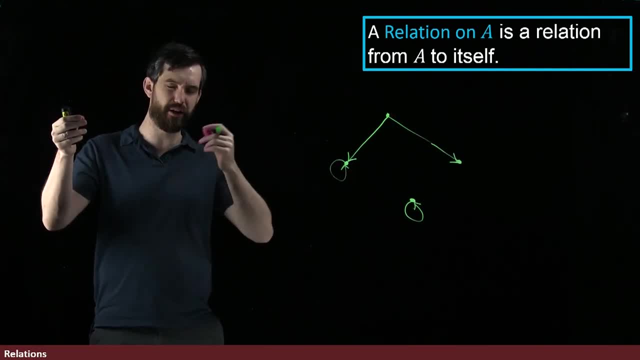 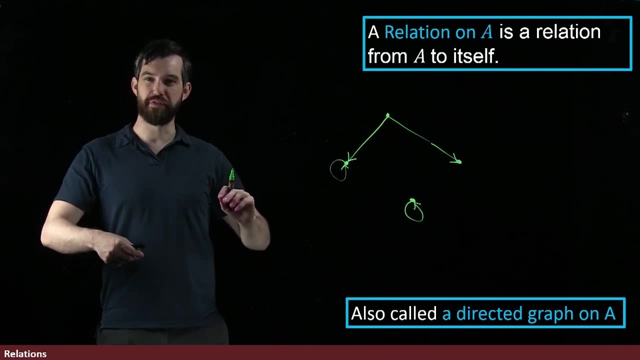 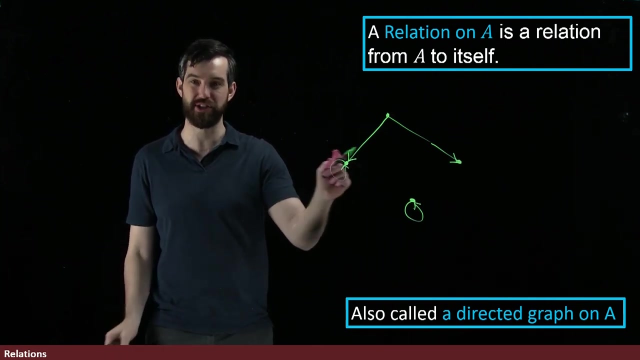 is a relation on A, an arrow diagram that starts on things in A and finishes on things in A. this is also referred to as a directed graph, where you've listed your various elements and then you draw directed arrows. Directed means has an arrow hat on it, just not just a connection between those. 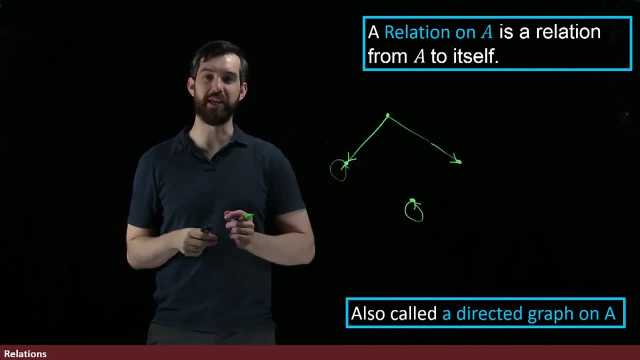 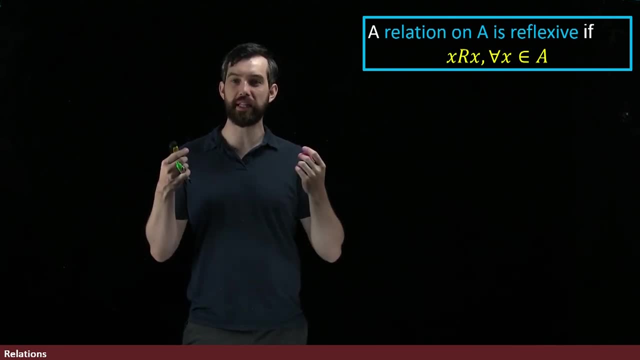 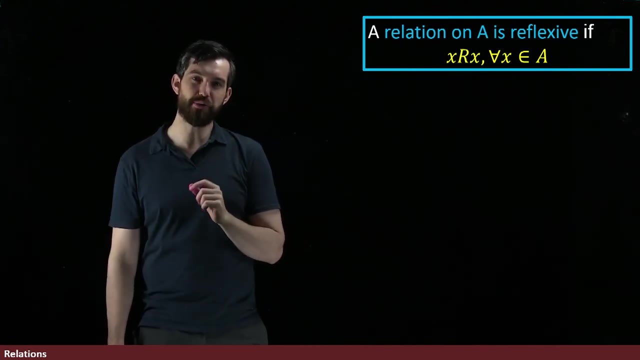 various elements and you get some graph between this set A. We then have a list of different properties that apply to relations on a set. One of them is this property of reflexive. So we're going to say a relation is reflexive if it relates to itself. 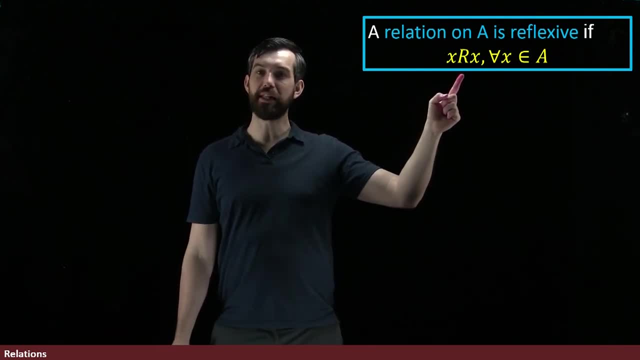 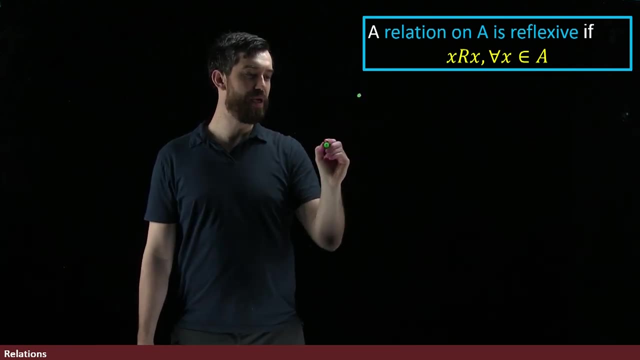 Or in other words, if X relates to X for all values of X inside of the A. So, for instance, if I was going to have maybe I'm just going to put three points here in my set. So this is a set with just three things in it. 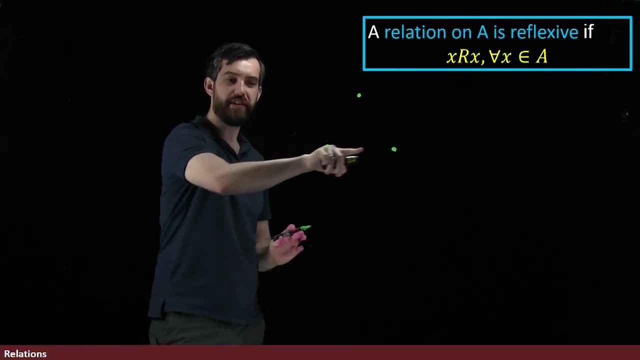 To claim it's reflexive means that any one of these three x values is related to itself, And related to itself means there's an arrow that starts there and finishes there, which is these little loopy things that I draw with an arrow on them. 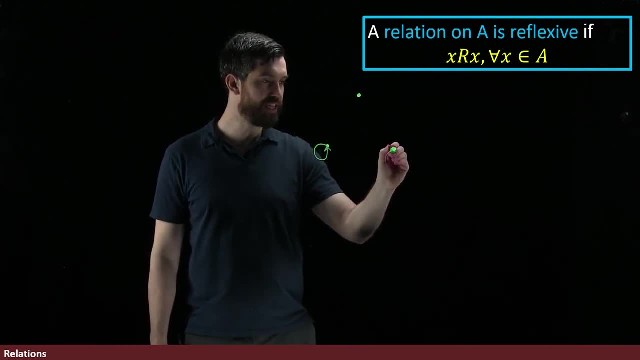 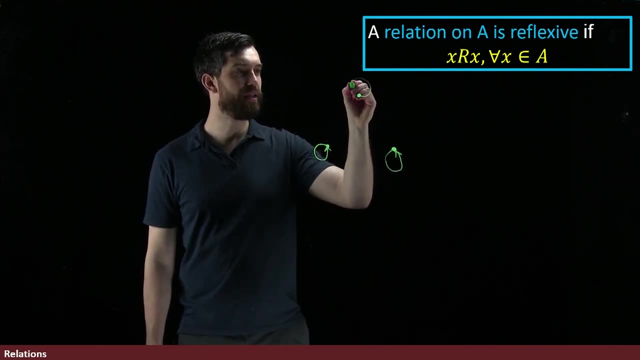 So this is saying that this point is related to itself. It's saying that this point is going to be related to itself, And it's going to say that this point is going to be related to itself as well. So all three points are related to themselves. 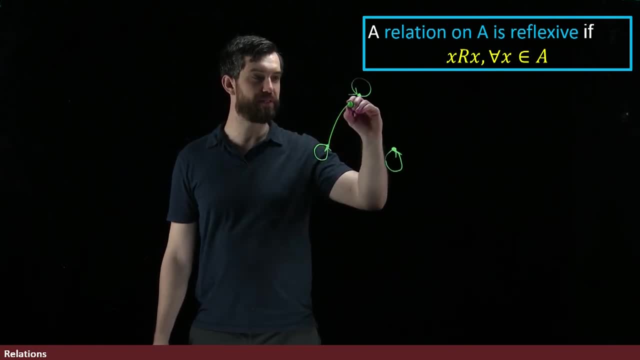 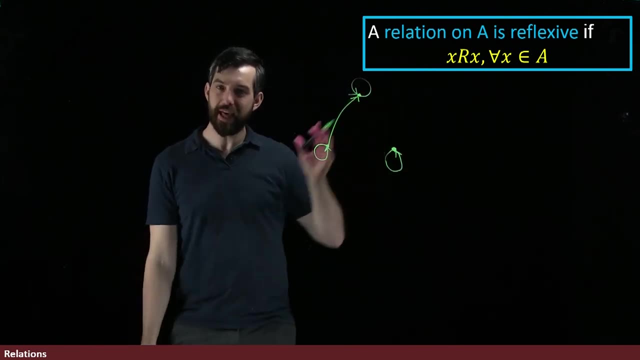 Now, it might be the case that there's other relations. Perhaps this particular one is related there, and maybe there's more, maybe there's not, But the other connections don't matter. To be reflexive, all that matters is that every point has one of these little loops around it. 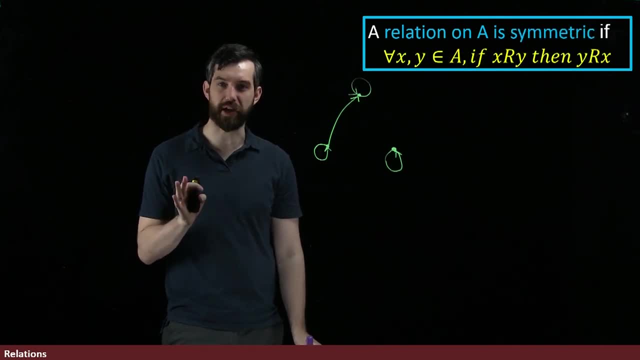 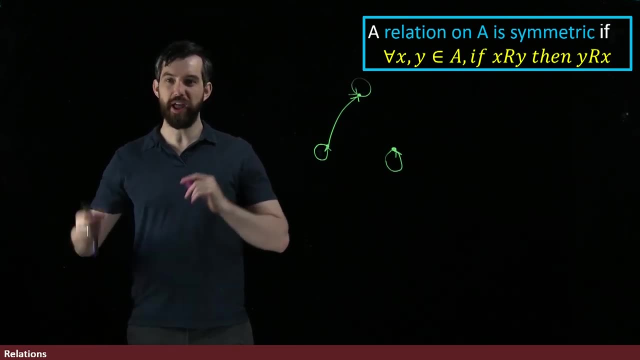 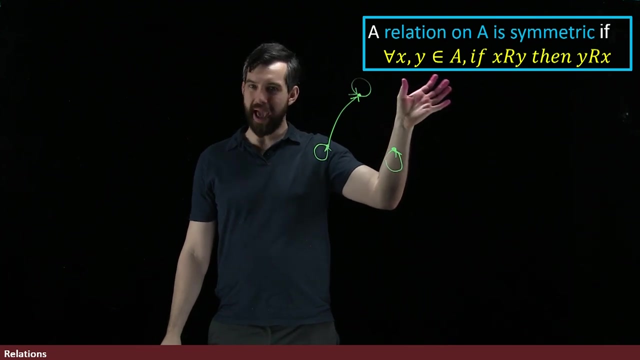 The next property we're going to talk about is called symmetric. So one of these relations on A is going to be symmetric if it has the following property: that if x were related to y, then y is related to x, Or in other words, for every pair that I might have, 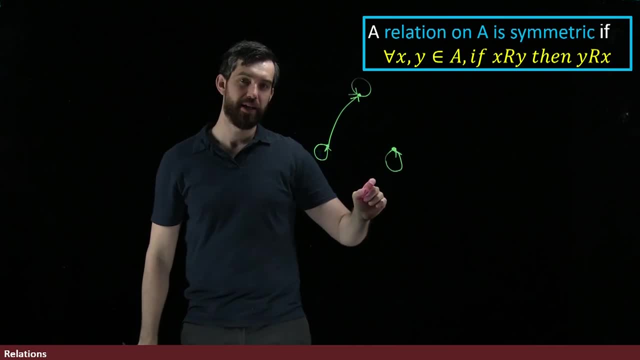 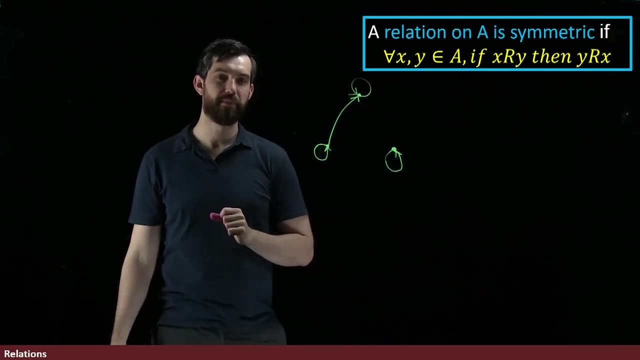 any two elements. how about these two elements here then? if there's a relation in the one direction, the x relates to the y, then the y relates to the x as well. As drawn this particular directed graph that I have, this relation on A is not symmetric. 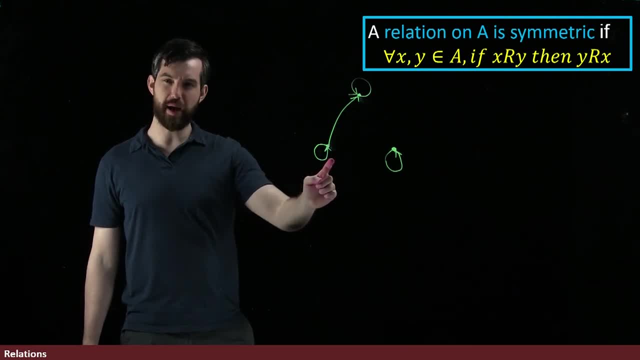 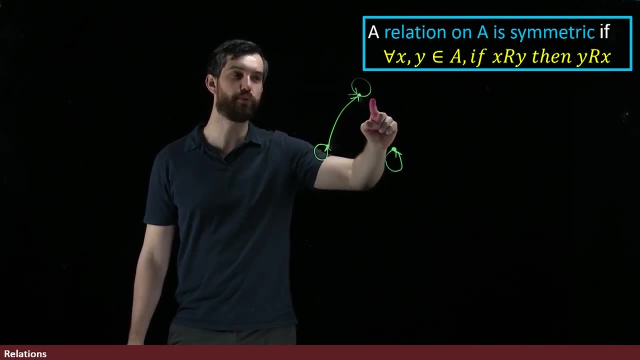 And it fails to be symmetric, because if this point here is my x and this point here is my y, then I have a relationship between x and y. x is related to y here because of this arrow connecting them, But y is not related to x because there's not. 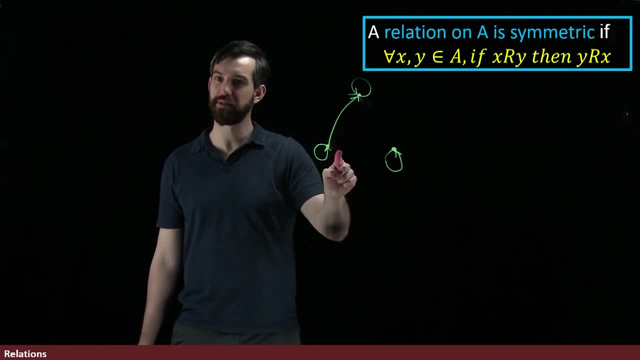 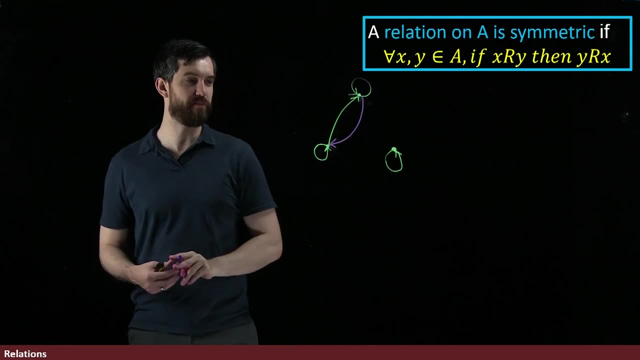 an arrow that starts at the y and finishes at the x. However, if I modify this and I came in and put an arrow like this, then it would become symmetric because the x, the y, x related to y and the y was related to x. 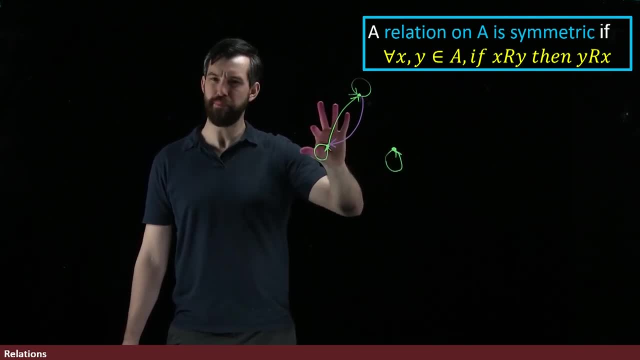 And note that the fact that this z that I have over here is completely disconnected doesn't matter, Because z isn't related to either the x or the y. I don't have to worry about there being a relation back. So the idea is this. 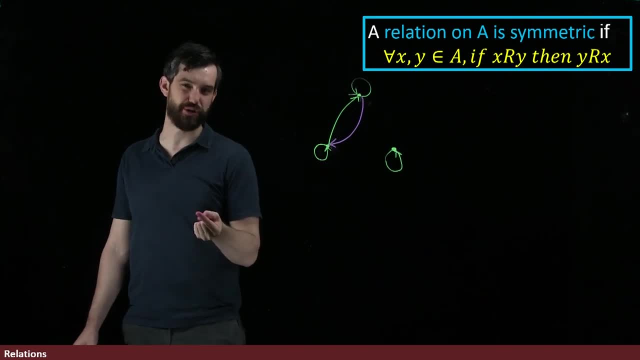 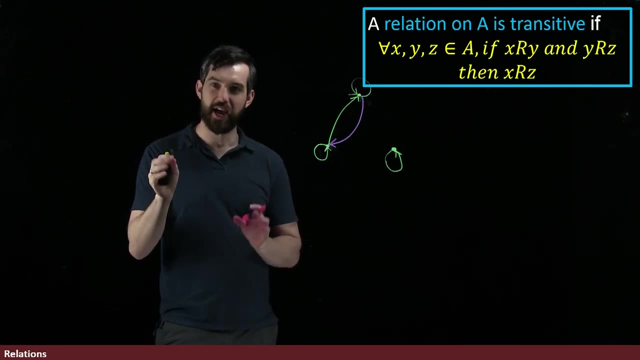 It is symmetric if every time you have an arrow in the one direction, it immediately turns around as an arrow coming right back. The final property that we're going to talk about is transitivity, And the idea here is this: Suppose it's the case that you've 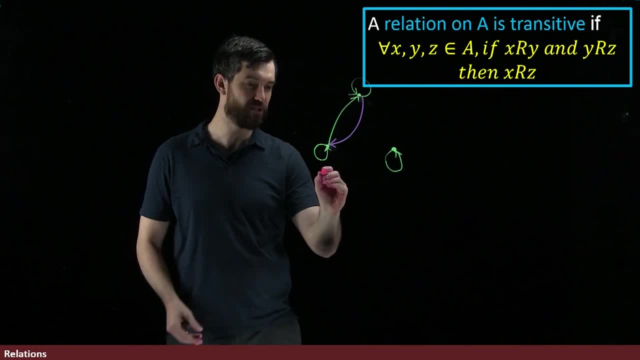 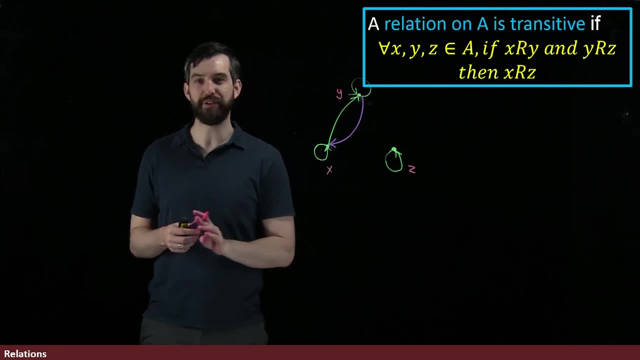 got three different points, And I've got an x, a y and a z. May as well label them here. I've got an x, I've got a y and I've got a z, And what you have is the following: 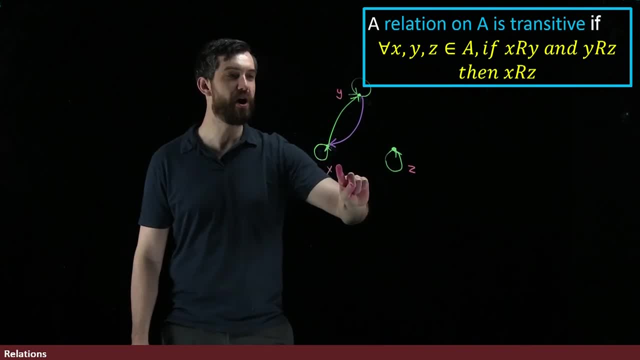 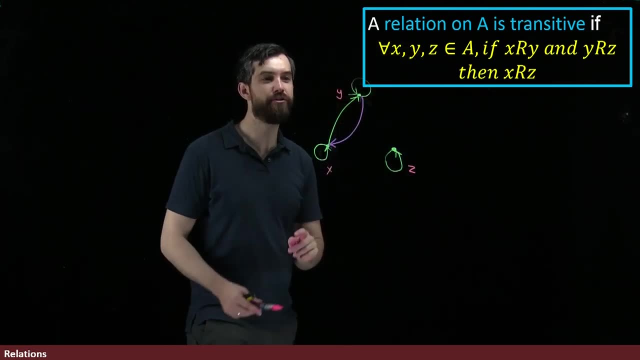 You've got that x is related to y. I've already got that x is related to y- good matches- And y is related to z. Well, I don't yet have that drawn in, so let me put it on. 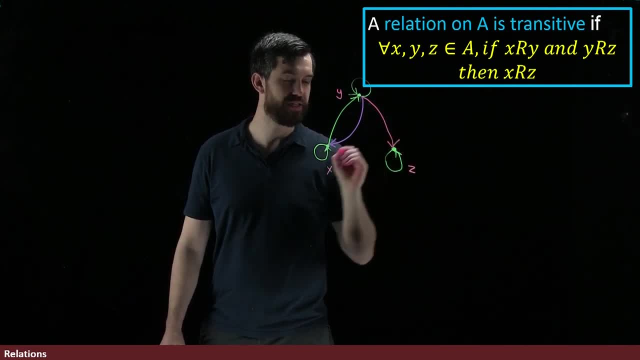 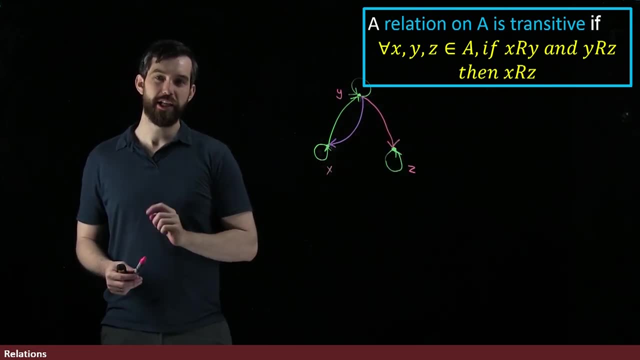 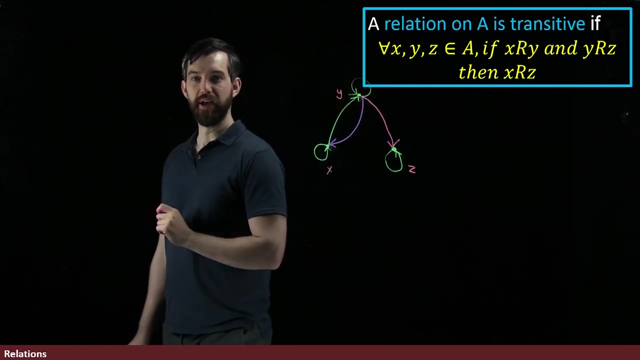 I'm going to say y is related down here to z, So x goes to y. I've got a relation there. y goes to z, I have a relation there. Then what I have is that x is directly related to z. So here's the idea. 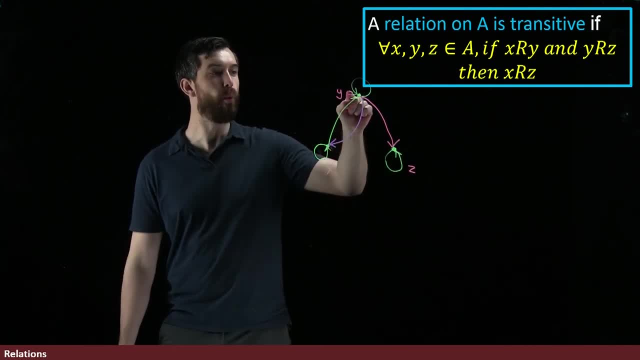 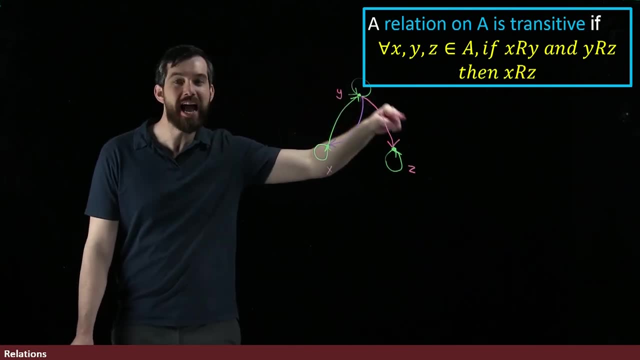 I can get from x to z in two steps. I can go from x to y along the green path and then y to z along the pink path, But if it's transitive, every time I can get to something by a long path. 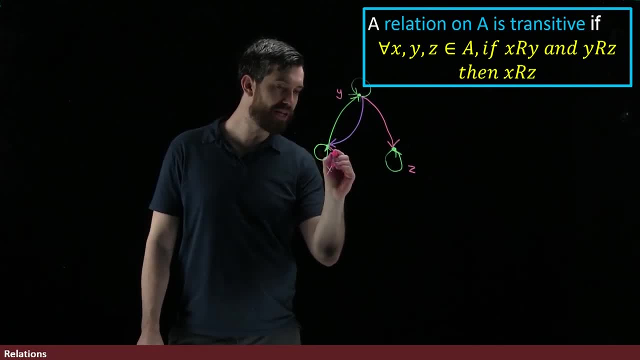 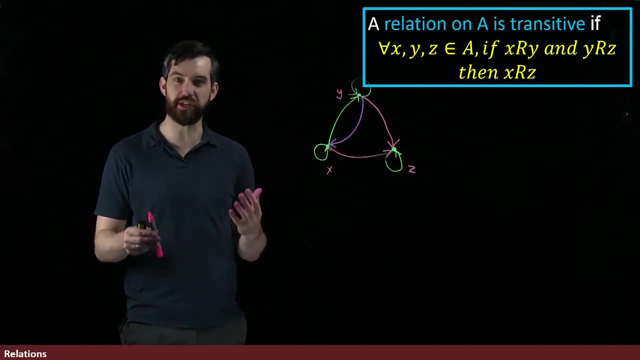 I can get there by a short one as well. I can go directly from my x to my y, And now this directed graph I have is transitive, because I can go from my x up to my y and then my y down to the z. 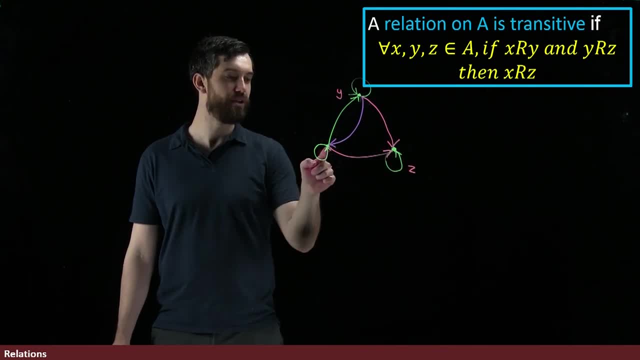 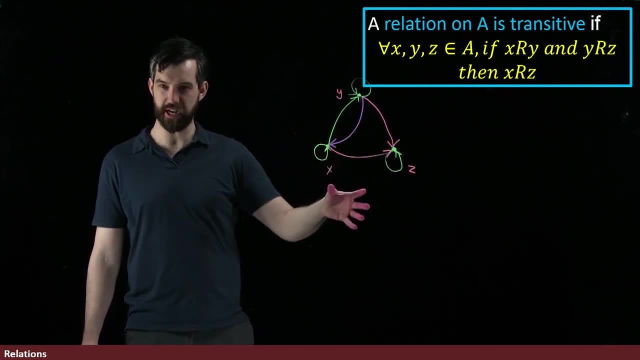 And when I have that cycle, I can then go directly from x to z. Note that there's also another loop that happens to be in here. from our previous descriptions Notice how the y was related to the x. I could go from y to x. 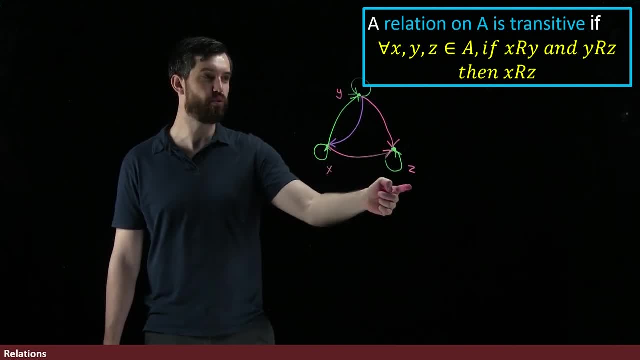 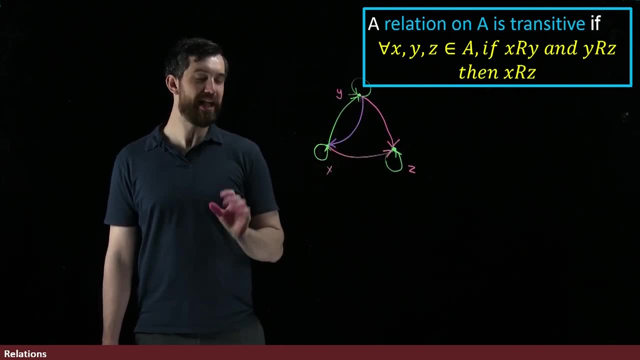 And then, from what we just wrote down, I can go from x to z as well. So there's a two-step path here. I can go from y to x and x to z, y to x and x to z, But I can also go directly. 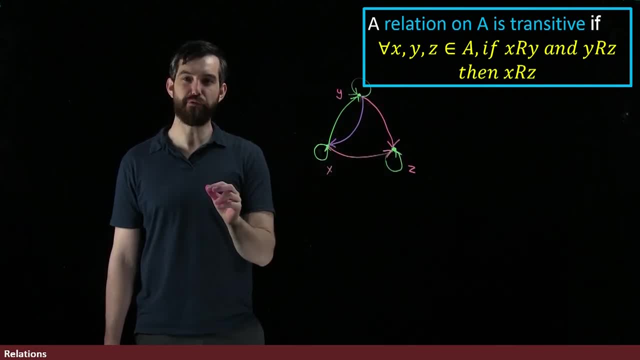 There's also a y to z path, So we've always got to be careful. As we start adding in more and more paths, there's more and more ways that it could fail to be transitive. So what you have to verify is that every way, 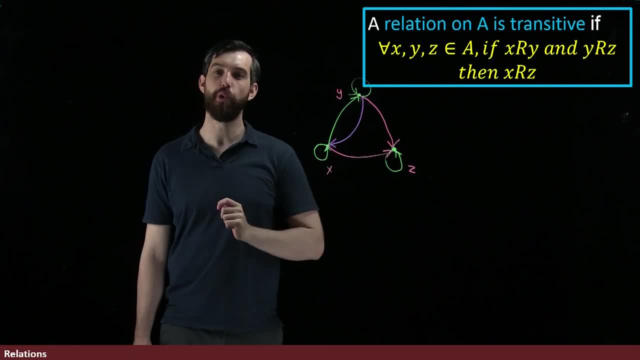 that you can get somewhere in a two-step path. you can get there in a one-step path as well. Thank you. 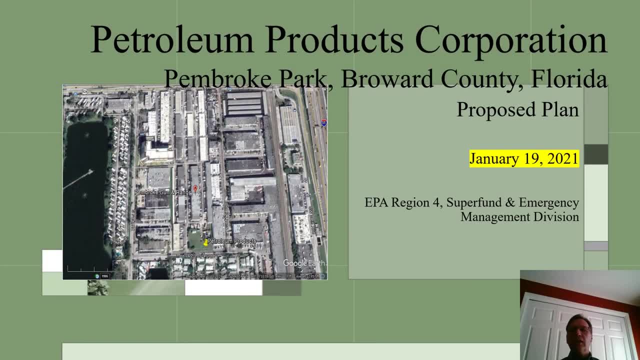 Welcome everyone. My name is Michael Taylor. I am a remedial project manager for the Environmental Protection Agency in Region 4.. I am here today to provide details on EPA's proposed cleanup plan for the Petroleum Products Corporation Superfund site, which I will refer to as the PPC site. 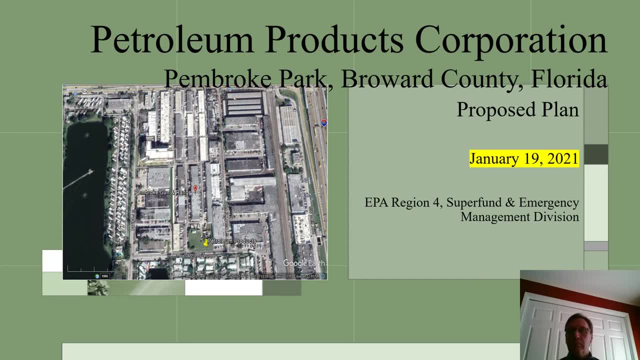 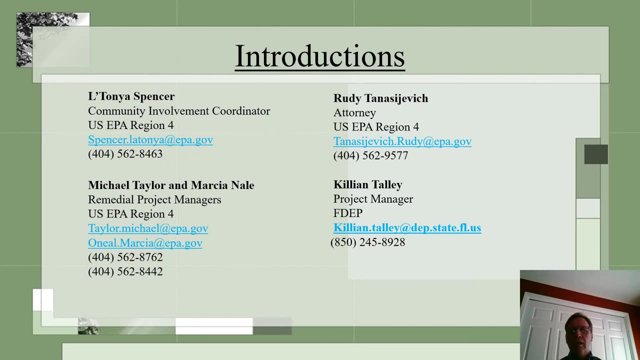 The PPC site is in Pembroke Park, Broward County, Florida. I will explain the history of the site, the Superfund process and how you can comment on our proposed cleanup for this site. Here you will find the contact names and numbers for EPA and the Florida Department of Environmental Protection that are associated with the site. 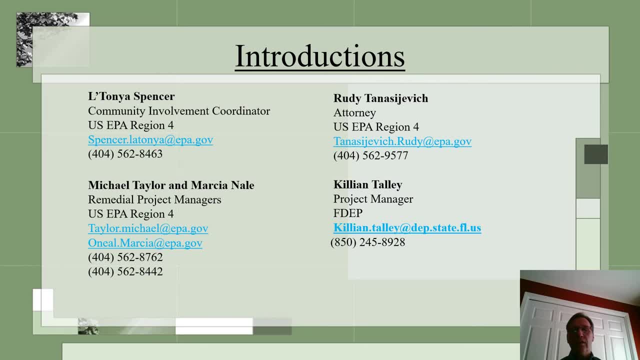 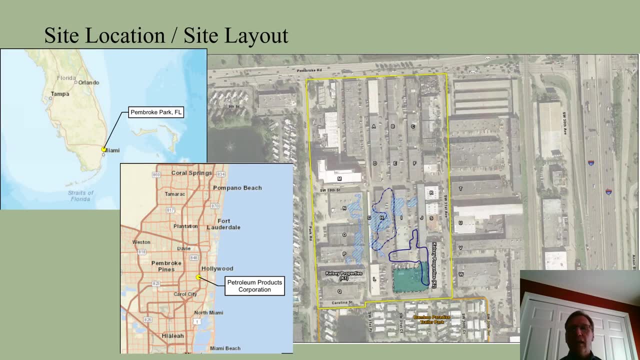 If you need further information after this presentation, we can be reached at the email and phone numbers provided. As I mentioned, the PPC site is located in Pembroke Park, between Fort Lauderdale and Miami. The former facility is located a quarter of a mile west of I-95, off of Pembroke Road. 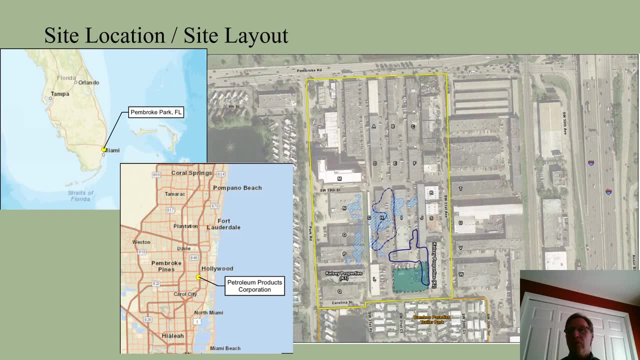 The yellow line in this figure indicates the approximate boundary and the area impacted for this Superfund site. It is approximately seven acres in size. There are multiple warehouses and storage units. currently on this property, Two former waste oil sludge pits that have been filled in exist. 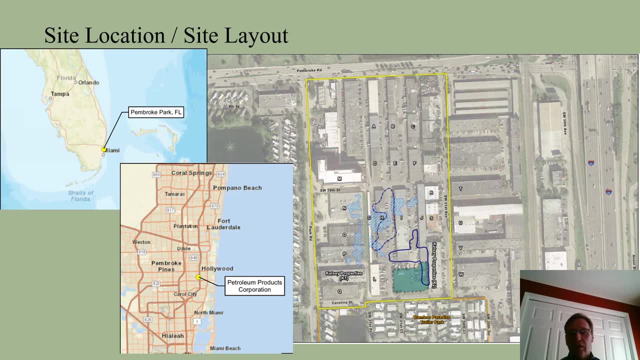 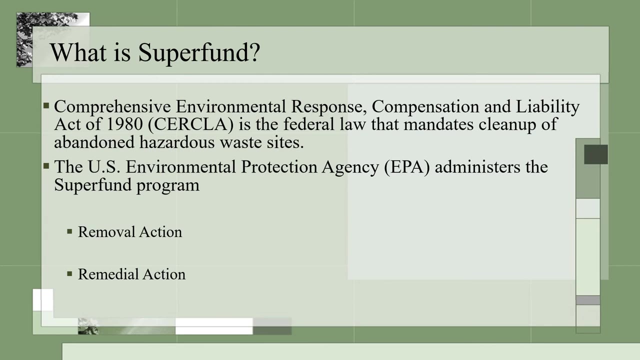 Underneath some of these structures, the contaminated soil and sludge has impacted the Biscayne Aquifer, which is a federally designated sole source aquifer. You have heard me mention the term Superfund. What is Superfund? This is a common name used in EPA for the Comprehensive Environmental Response Compensation and Liability Act, or CERCLA. 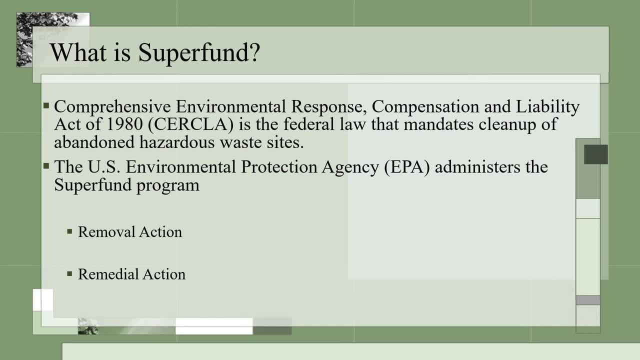